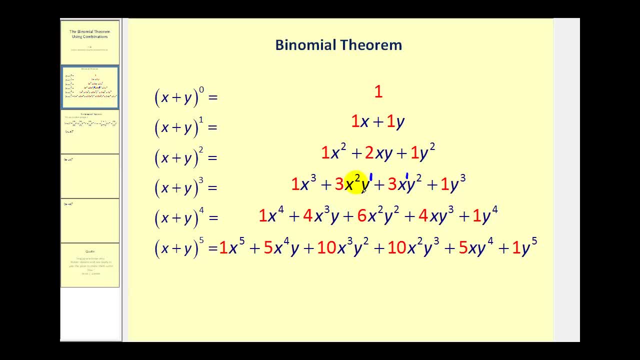 three, The third term, we have x to the first. so the factors of x has dropped by one again and we've picked up another factor of y all the way to y to the third. So if we jump down to the quantity x plus y to the fifth notice, we have x. 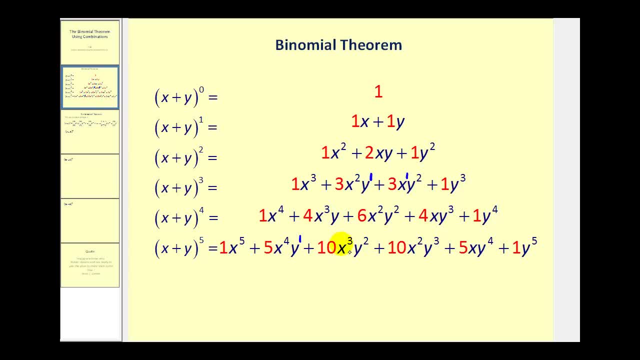 to the fifth, then x to the fourth, y to the first, x to the third, y to the second, and so on. So as we go from left to right, we lose factors of x's and pick up factors of y. Next in red we have these coefficients that we found last time. 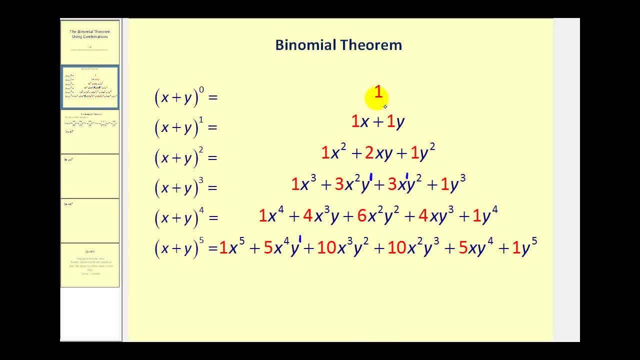 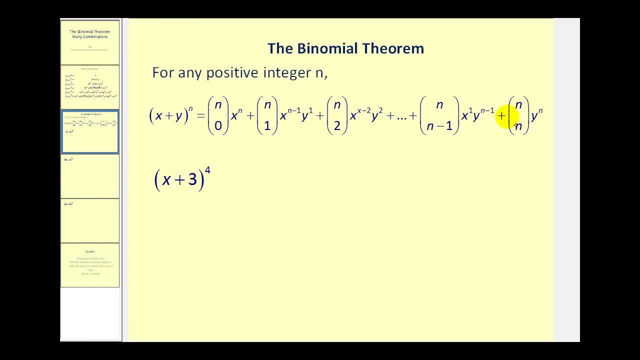 using Pascal's triangle, but now we'll take a look at how we can find them using combinations. Let's go and take a look at the binomial theorem. So this can look a little intimidating, but again, the idea here is to recognize the pattern. 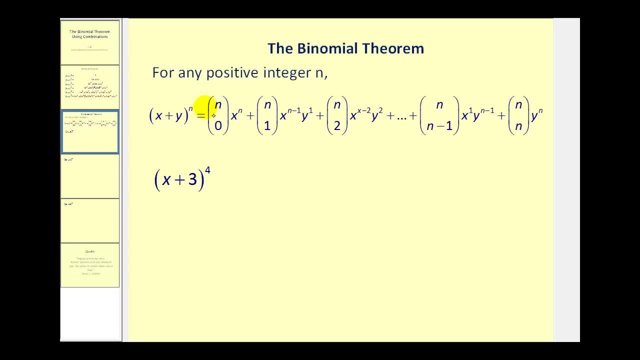 Notice: the exponent on x in the first term matches the original exponent. and then we decrease the factors of x by one and start picking up factors of y, And then those red coefficients on the previous screen can be found from these combinations: n choose zero, n choose one, n choose two all the way to n choose n. 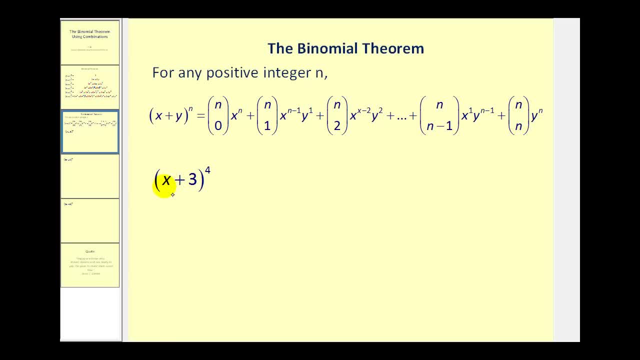 Let's see if we can apply that to expand the quantity x plus three to the fourth power. Let's first write out the variable part and then we'll come back and find the combinations. So the first term would be x to the fourth and zero factors of. 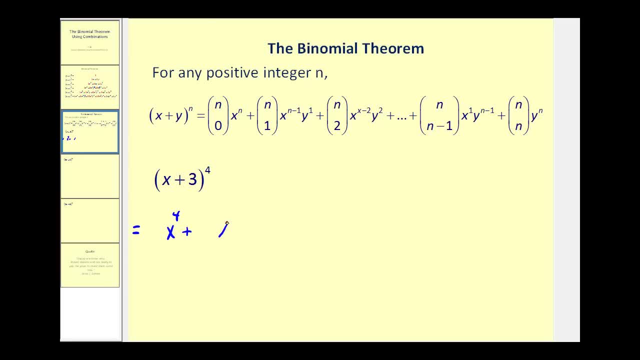 three. plus then we'd have three factors of x and we'd start picking up factors of three. Notice that instead of y we have three, but the process is going to be the same. Plus now we'll have two factors of x and two factors of three, plus one factor of. 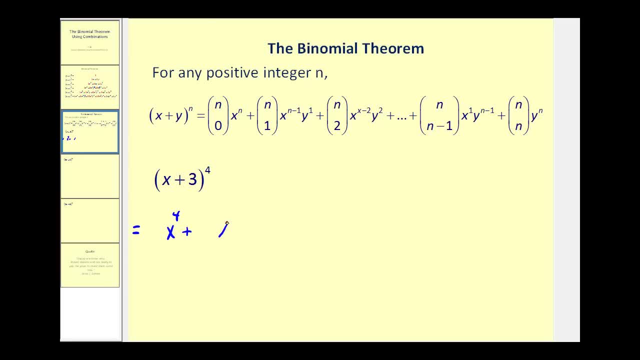 three. plus then we'd have three factors of x and we'd start picking up factors of three. Notice that instead of y we have three, but the process is going to be the same. Plus now we'll have two factors of x and two factors of three, plus one factor of. 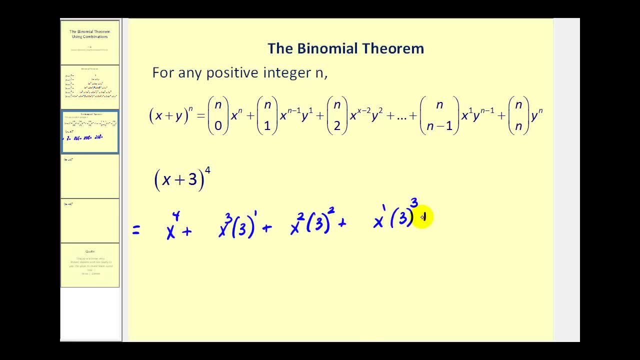 x and three factors of three. and lastly, we have zero factors of x and four factors of three. So now to find the missing factors. here we'll start finding combinations. This first one will be n- choose zero. or four, choose zero. The second will be four, choose one. We'll continue this. 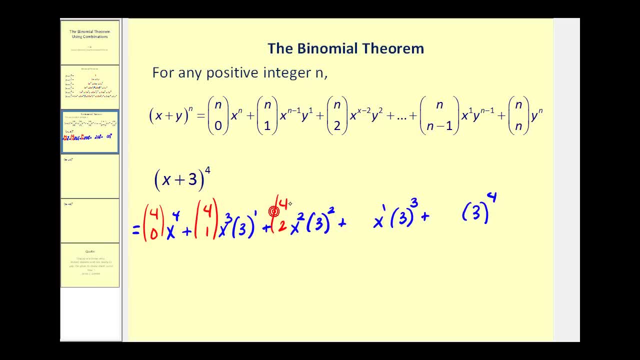 all the way out to four choose four. So when we find these products, this will be the expansion of this binomial. Let's go and show a little more work here. Four choose zero. 4 choose 0 would be 4 factorial over n minus r factorial, that's 4 factorial and then 0 factorial times x to the 4th. plus 4 choose 1 would be 4 factorial 3 factorial 1 factorial times x to the 3rd. times 3 plus 4 choose 2 would be 4 factorial 2 factorial 2 factorial x to the 2nd. 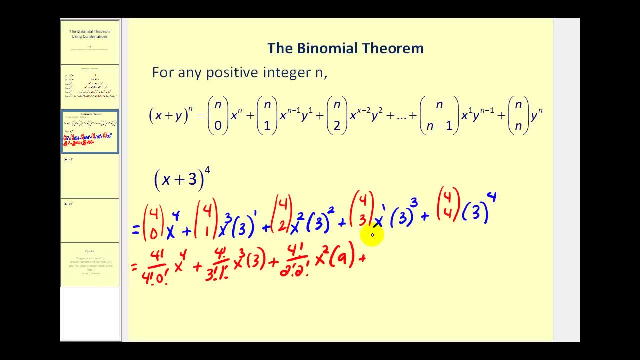 3 squared, that would be 9 plus 4 choose 3, that's 4. factorial 1. factorial 3. factorial notice that 4 choose 1 and 4 choose 3 are the same x, and then 3 to the 3rd, that would be 27. and then, lastly, 4 choose 4, that's going to be the same as 4 choose 0, 4- factorial 0. factorial 4. factorial times: 3 to the 4th, that's going to be 81.. 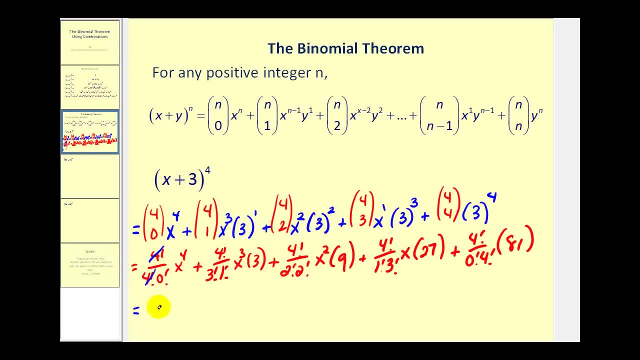 So this would be equal to 1.. So we have x to the 4th, 4 factorial over 3 factorial, that's going to be 4, and 1 factorial is 1, so we have 4 times 3, that would be 12x cubed, plus 4 factorial over 2 factorial, 2 factorial- well, 2 factorial times 2 factorial would be 4, so this would equal 6 times 9,, that's 54x squared plus this is equal. 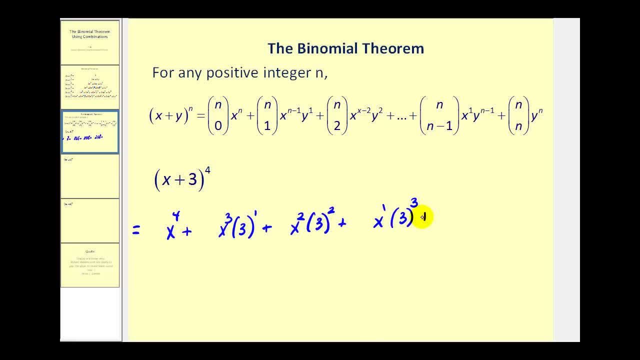 x and three factors of three. and lastly, we have zero factors of x and four factors of three. So now to find the missing factors. here we'll start finding combinations. This first one will be n- choose zero. or four, choose zero. The second will be four, choose one. We'll continue this. 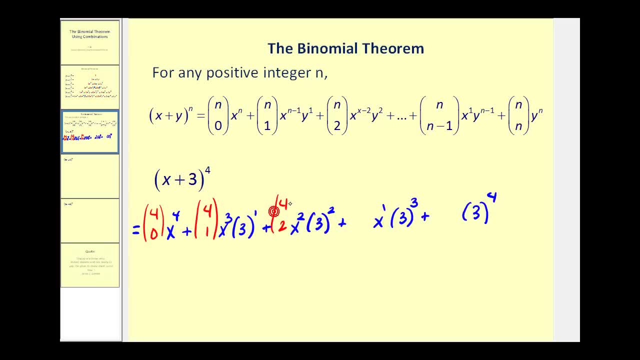 all the way out to four choose four. So when we find these products, this will be the expansion of this binomial. Let's go and show a little more work here. Let's go ahead and show a little more work here. Four choose zero would be four factorial over n minus r factorial, That's four factorial and then. 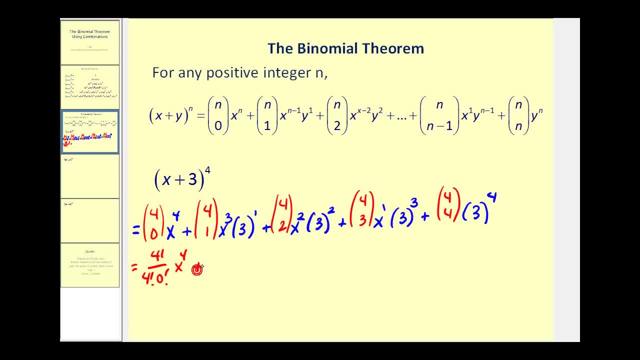 zero. factorial times x to the fourth plus four. choose one would be four. factorial three. factorial one. factorial times x to the third, times three plus four. choose two would be four. factorial two factorial two. factorial X to the second: three. three squared, that would be nine plus. 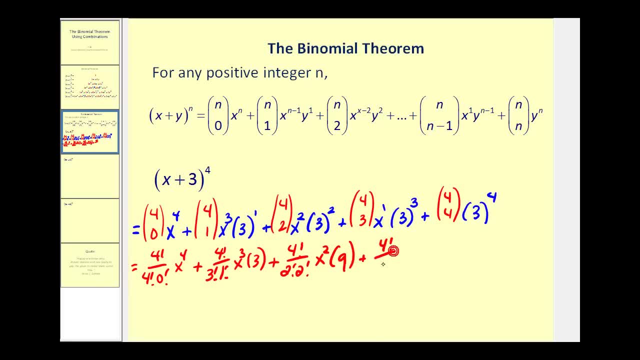 four choose three. that's four factorial one, factorial three, factorial. Notice that four choose one and four choose three are the same X, and then three to the third, that would be twenty-seven. And then, lastly, four choose four. that's going to be the same as four choose zero. 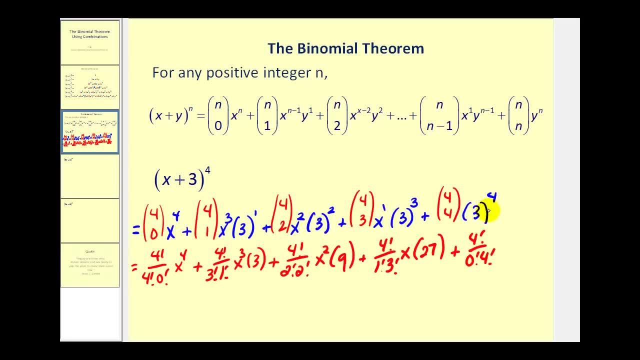 Four factorial zero factorial. four factorial Times: three to the fourth, that's going to be eighty-one. So this would be equal to one. so we have x to the fourth. Four factorial over three factorial, that's going to be four. 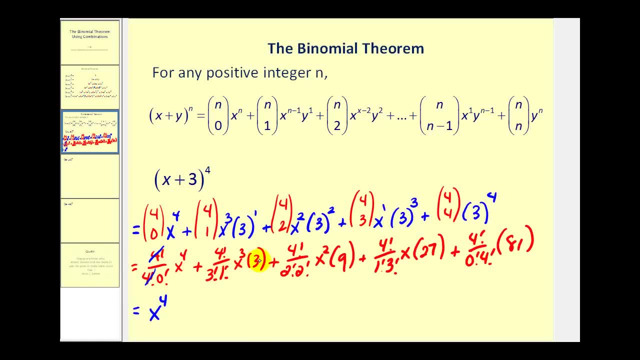 And one factorial is one. so we have four times three, that would be twelve x cubed Plus four factorial over two factorial, two factorial. Well, two factorial times two factorial would be four. So this would equal six times nine, that's. 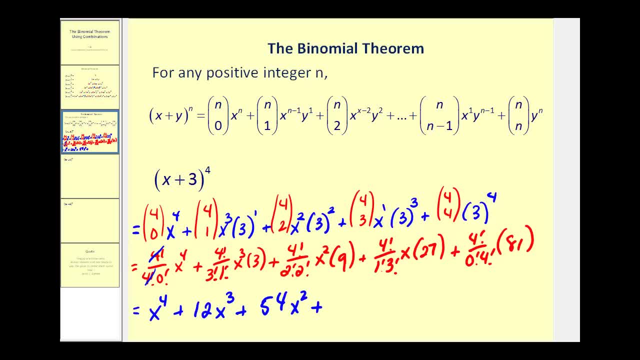 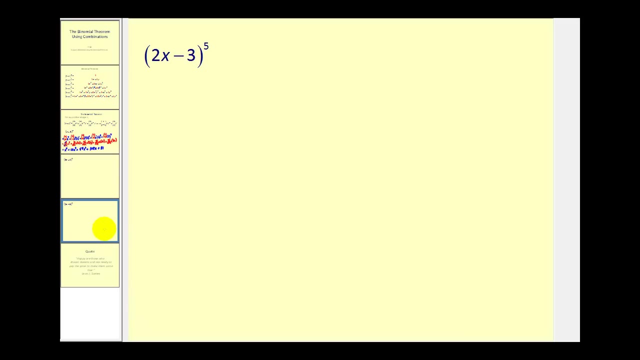 fifty-four x squared Plus, this is equal to four times x. times twenty-seven, that's one hundred eight x. And then, lastly, we have: this is equal to one times eighty-one. so we have eighty-one. Let's go and take a look at another one. 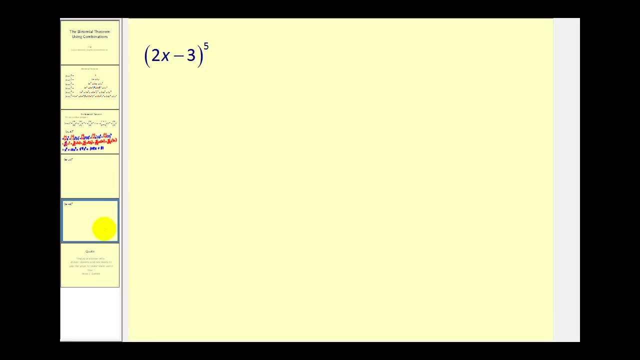 Here we have the quantity two x minus three raised to the fifth power. So again, let's first write out the patterns with these two terms and then we'll write in the combinations to find the missing factors. So for the first term we'd have two x to the fifth plus 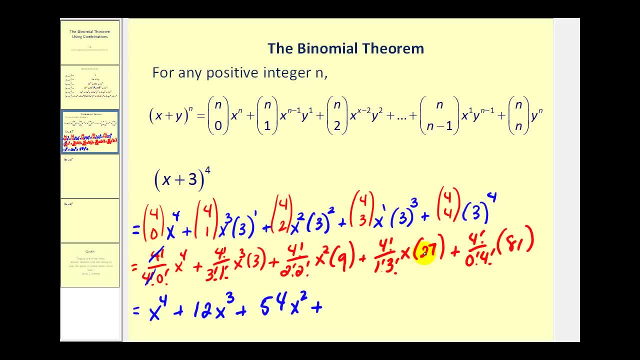 to 4 times x, So we have 4 times 6 times 27,, that's 108x. and then, lastly, we have: this is equal to 1 times 81,, so we have 81.. Let's go and take a look at another one. 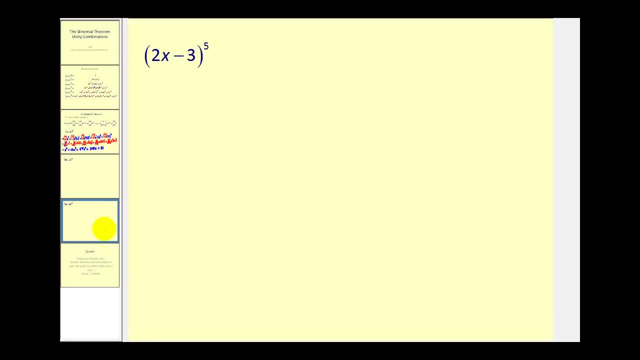 Here we have the quantity 2x minus 3 raised to the 5th power. so again, let's first write out the patterns with these two terms and then we'll write in the combinations to find the missing factors. So for the first term we'd have 2x to the 5th plus, and then we'll lose one factor of 2x. 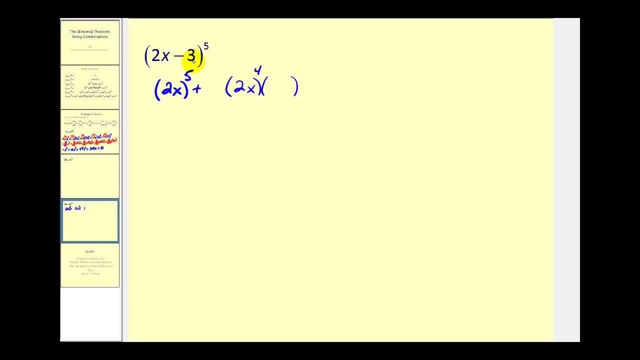 So we'll put 2x to the 4th. Now the second factor is going to be negative 3, because we have a minus 3 here. Remember we could write this as 2x plus negative 3.. So we have a negative 3 to the power of 1 plus 2x to the third, negative 3 to the second plus 2x to the second. 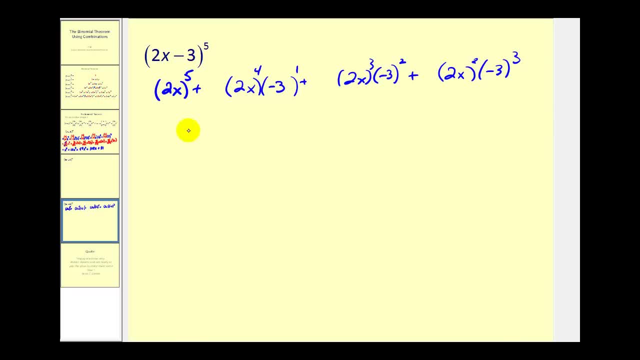 negative three to the third, We'll have to go down to the next line. now We have plus. this would be two x to the first and negative three to the fourth. Remember these are always adding to five. Then we have one more term here. 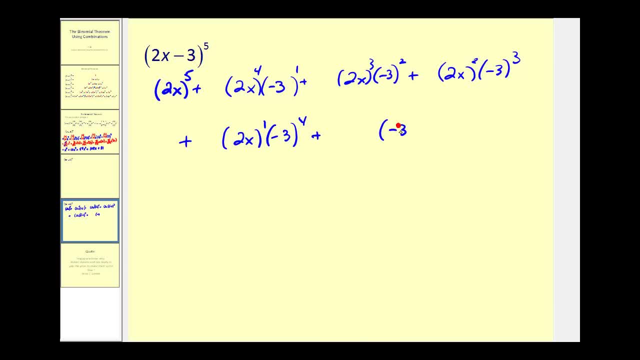 It's going to be two. x to the zero power, that's one. Then we have negative three to the fifth power. To find the missing factors, in front we'll find combinations. This will be five, choose zero. This will be five, choose one. 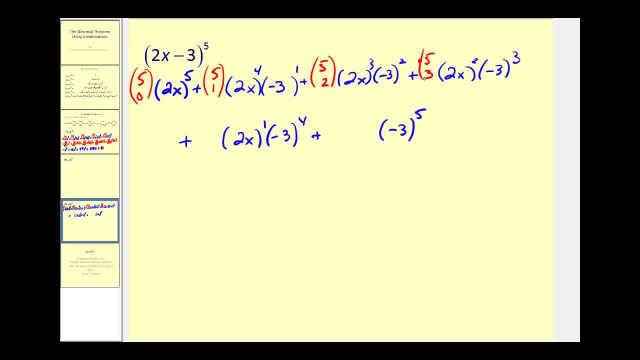 Five choose two, And you see the pattern. Now we just have to find the values of these combinations and then find the products. Five choose zero is one, So one times two to the fifth, that would be 32 x to the fifth. 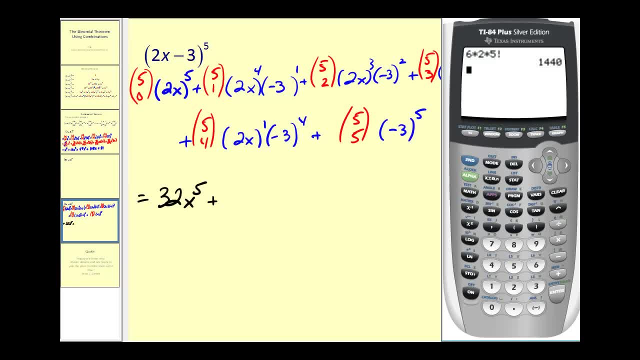 Plus, let's go ahead and use our calculator now: Five choose one is equal to five, So we have five five times. we have a factor of negative three, And we also have four factors of two, two to the fourth, So it's negative 240,. 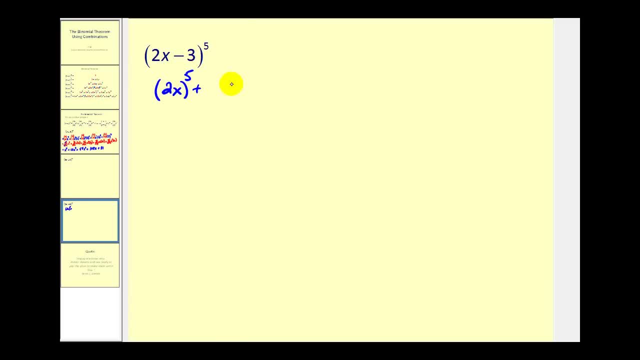 and then we'll lose one factor of two x, So we'll have two x to the fourth. Now the second factor is going to be negative three, because we have a minus three here. Remember we could write this as two x plus negative three. 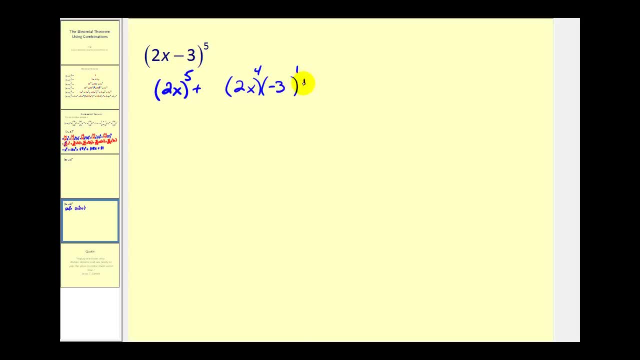 So we have a negative three to the power of one plus two x to the third, negative three to the second plus two x to the second, negative three to the third. We'll have to go down to the next line. now We have plus. 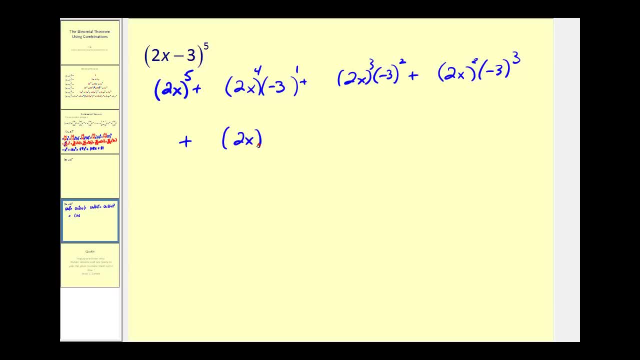 this would be two x to the first and negative three to the fourth. Remember, these are always adding to five And we have one more term here. It's going to be two x to the zero power. that's one. Then we have negative three to the fifth power To find the. 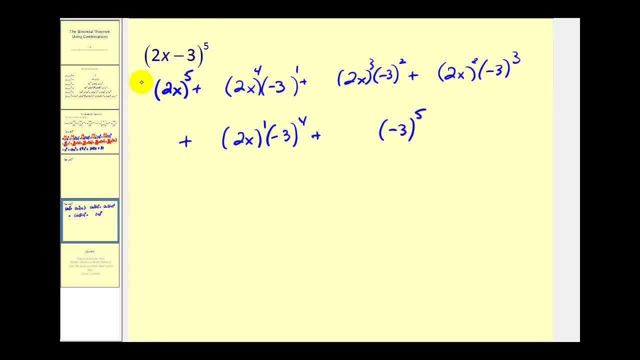 missing factors. in front we'll find combinations. This will be five choose zero. this will be five choose one, five choose two, and you see the pattern. Now we just have to find the values of these combinations and then find the products. Five choose zero is one. 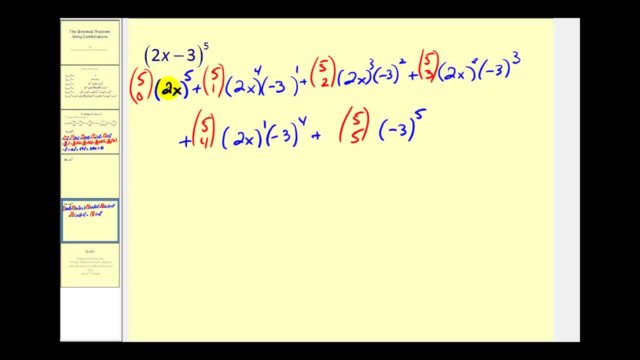 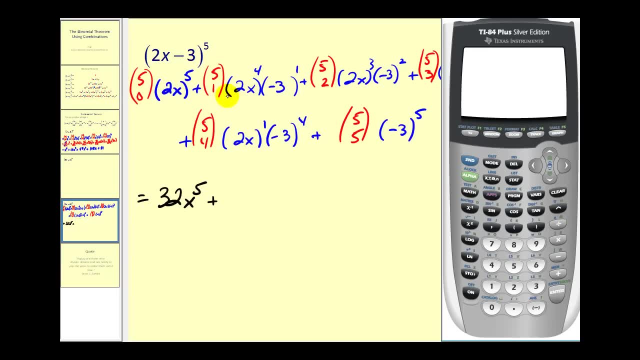 So one times two to the fifth, that would be thirty-two x to the fifth, plus let's go ahead and use our calculator now: Five choose one is equal to five, So we have five times we have a factor of negative three. 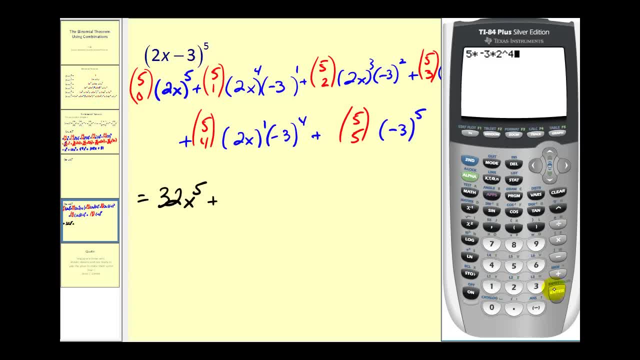 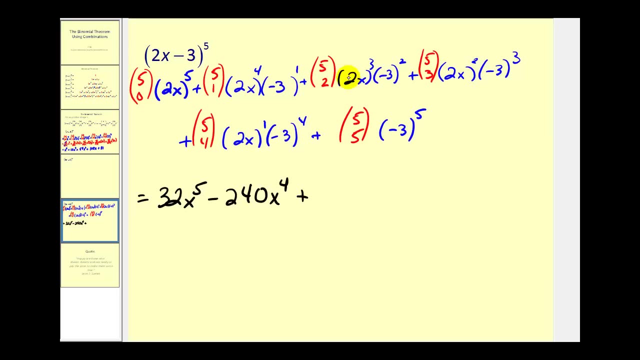 and we also have four factors of two. two to the fourth, So it's negative two hundred forty. so this will be negative two hundred forty x to the fourth. So we'll write this as minus two hundred forty x to the fourth. Next we're going to have five. choose two. 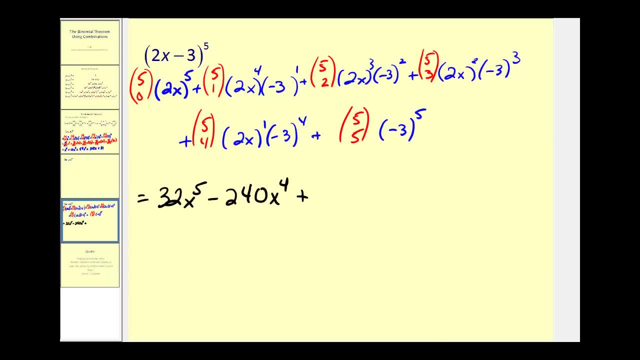 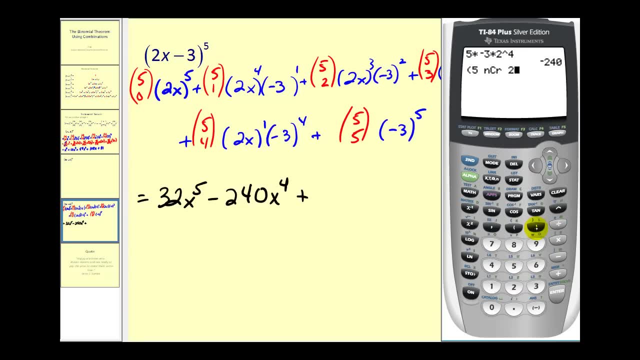 times this would be two to the third times negative three squared. So we have five. option three, so five. choose two times two to the third times negative three squared, which would be nine. So we have seven hundred twenty and this would be x to the third. 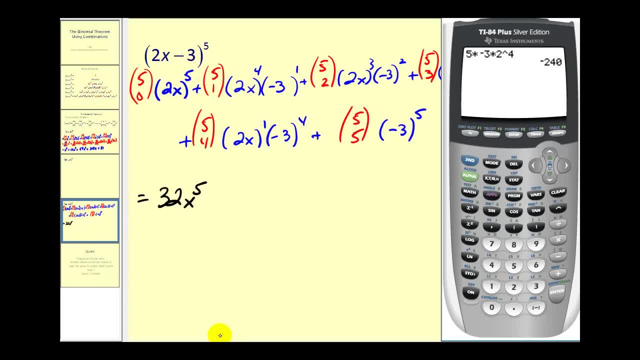 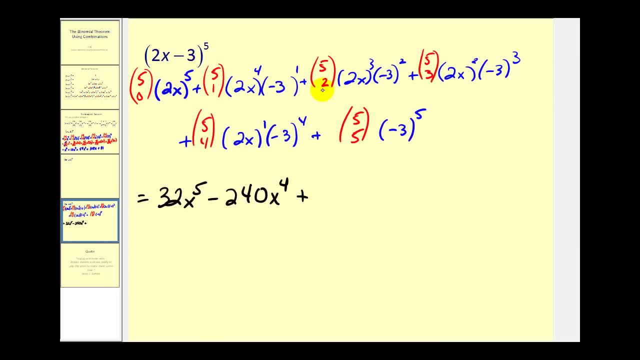 so this will be negative 240 x to the fourth. So we'll write this as minus 240 x to the fourth. Next we're going to have five. choose two times. this would be two to the third times, negative three squared.